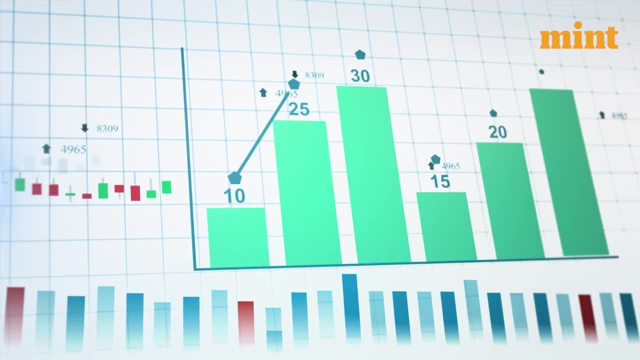 Robin Chhabra, founder and CEO of Dextrous Workspace, said that the year 2023 could be interesting, As we observe an increase in GDP per capita, higher disposable incomes, expanding urbanization. As we observe an increase in GDP per capita, higher disposable incomes, expanding urbanization. 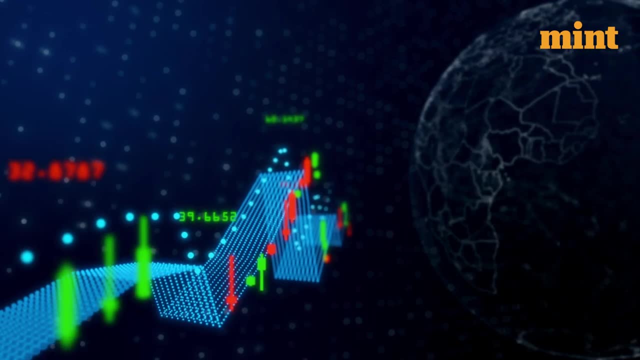 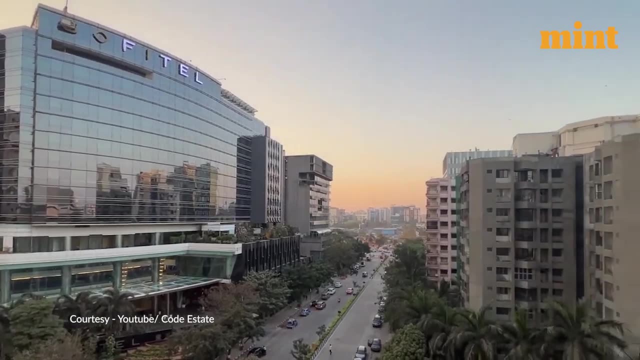 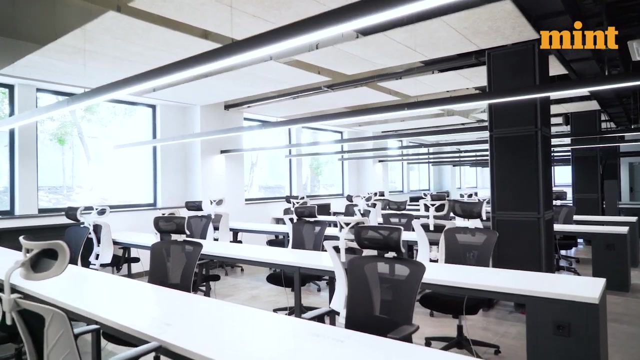 and, most importantly, a greater focus on us as the next major economy, The real estate sector will continue on its path of long-term expansion. It would be interesting to know that offices and commercial space would be in high demand in Tier 1 and Tier 2 cities. 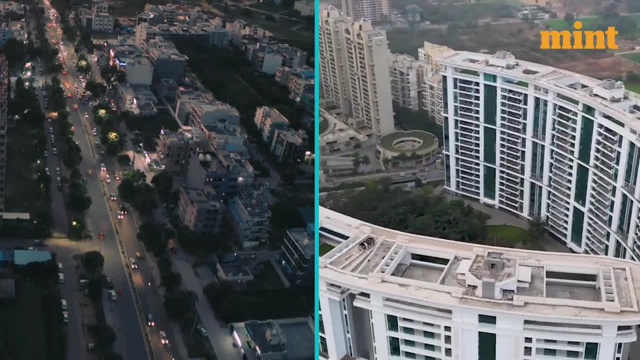 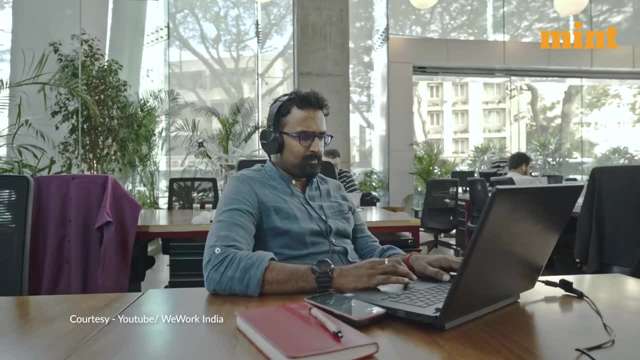 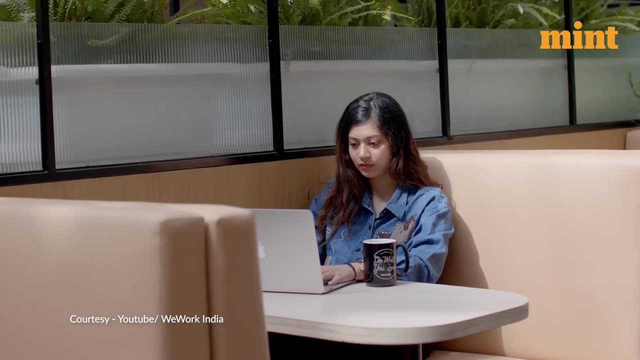 This means that the commercial development in cities like Pune, Hyderabad, etc. will be on the rise. The co-working sector will continue to rise and by the end of 2023, it is predicted to reach 50 million square feet, a rise of 15% year-over-year. 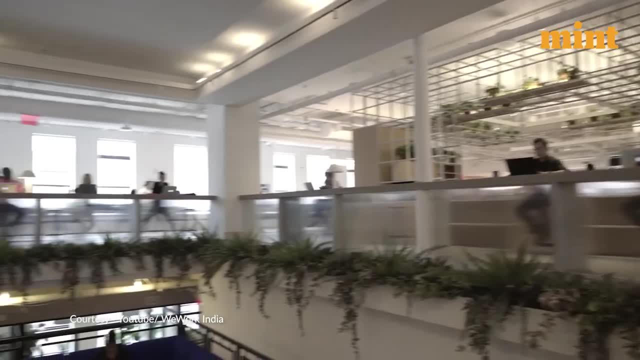 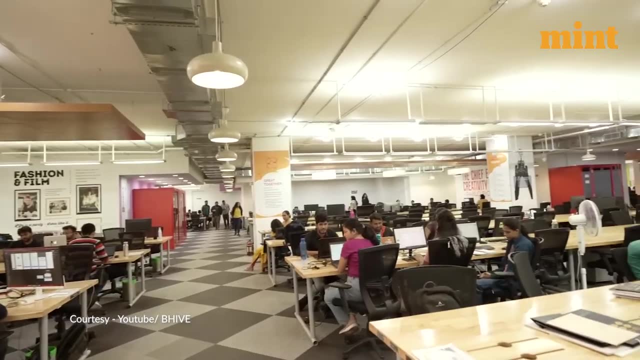 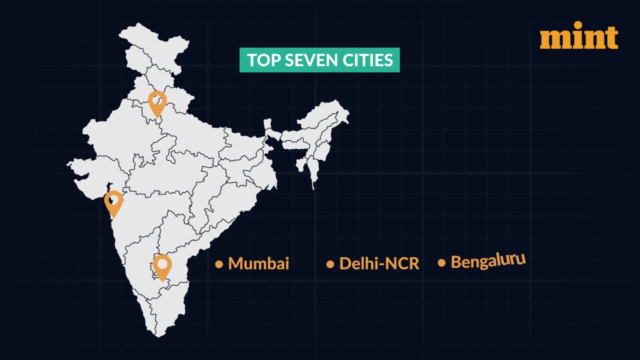 Apart from this, the managed office spaces will also continue to grow at 10% in 2023.. As per the recent JLL report, the net absorption of office space in 2022 across the top 7 cities like Mumbai, Delhi, NCR, Bengaluru, Hyderabad, Chennai. 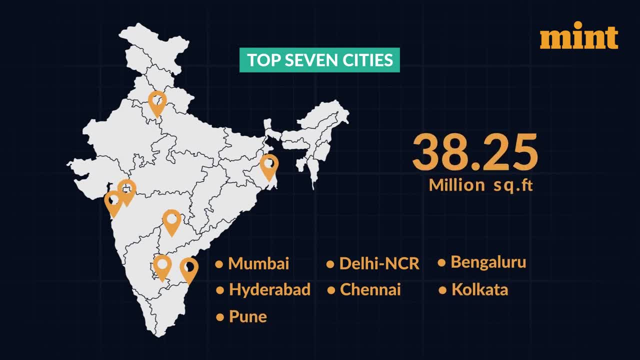 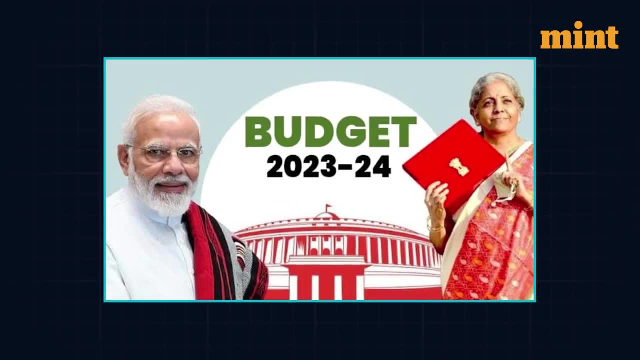 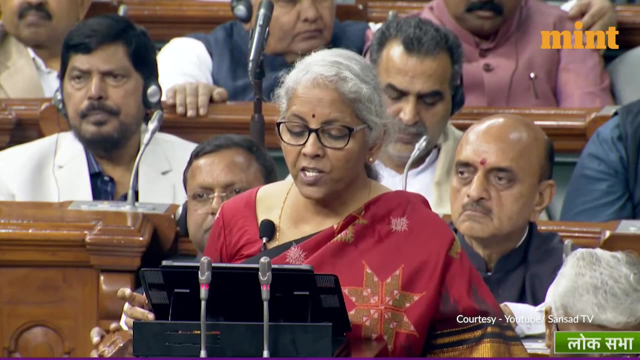 Kolkata and Pune has been 38.25 million sq ft. Mr BL Narayana, CEO and founder of Nesca Homes, said that the Union Budget 2023-24 is remarkable for the real estate sector. The Finance Minister has announced green growth as one of the priorities of the budget. 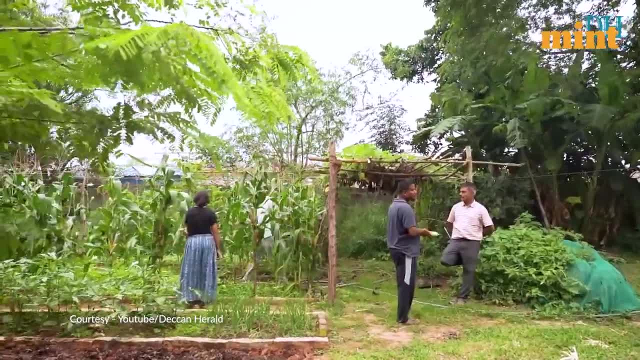 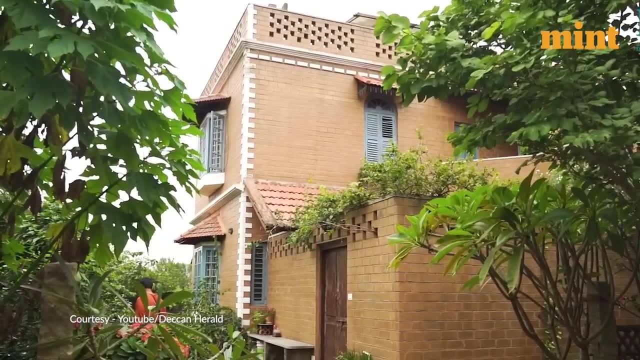 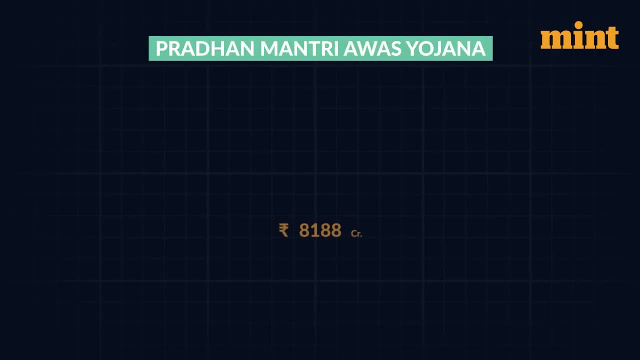 Many firms that are working towards green and sustainable living are helping to achieve these goals more efficiently. With environmental challenges, this move towards sustainable infrastructure will help in welcoming a brighter future. Apart from this, the Pradhan Mantri Awas Yojana allocated Rs 79,000 crore for affordable housing. 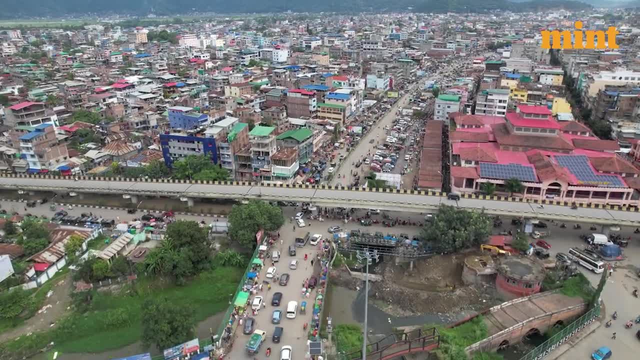 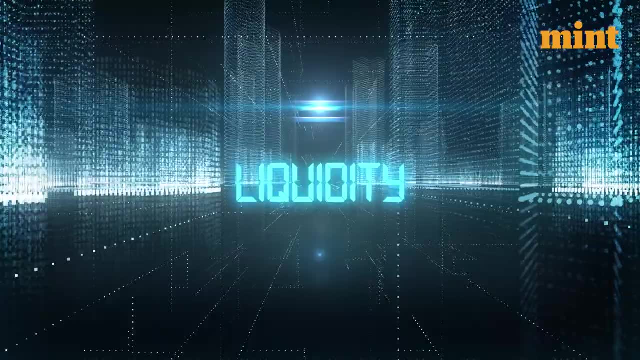 If we consider the current domestic and international scenarios, the budget is holistic and growth-oriented. Higher tax debates will undoubtedly increase market liquidity, resulting in more disposable income. That is why we are looking forward to the future. That would encourage people to buy properties.